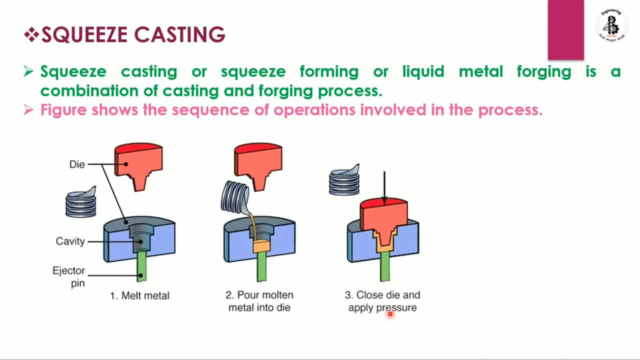 apply the pressure. So that will be similar kind of arrangement, just you can applying the forging, So with the application of that particular force, or you can say pressure with the help of die, towards the molten form of the metal which will be filled into a mold cavity. So this is our material and with the application of pressure, it will be applying the pressure. Then on to the last steps. 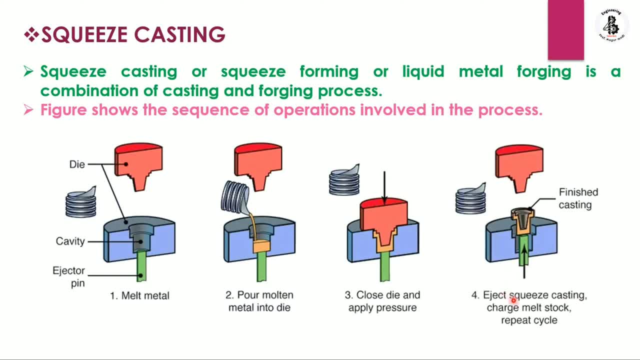 after the solidification process, just eject the squeeze castings, charge metal stocks and repeat the cycles. Or you can say in simple way: after removing the pressure, with the help of die, just you can see, with the help of ejector pin, you will get a finished casting process. So basically, into these squeeze casting process, or you can say squeeze forming, or you can say forging process, So that 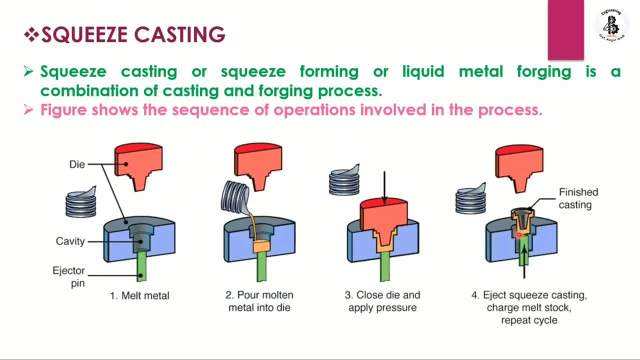 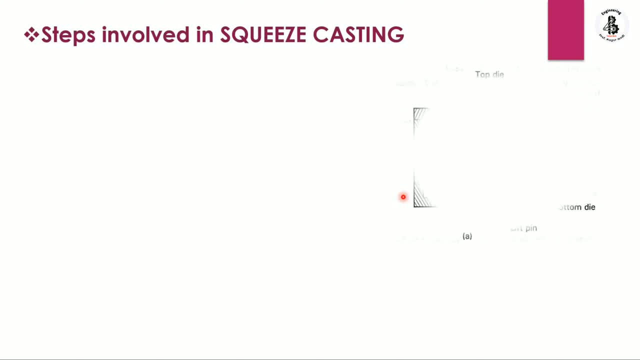 are used to know as a combination of the all that processes. So basically, just you can see the various steps that will be involving. So this is our cavity, this white color, This is our bottom die and this one is our top die, or you can say punch. So, as from my shape and size of our job, I would like to make a bottom die. 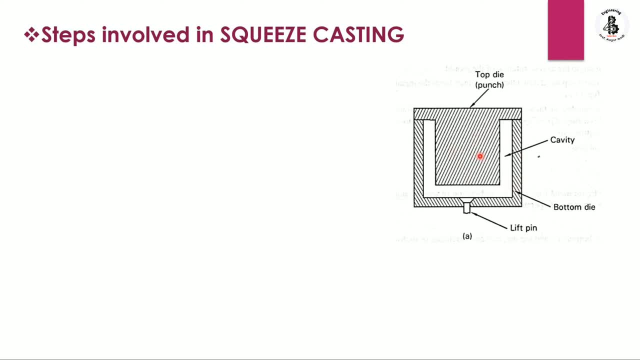 die as well as the top punch die and in between it will be my required shape and size. or you can say cavity and at the, and just you can see, this is our ejector pin. or you can say lift pin, so after the solidification process, that will be used to ejecting the components. so just you can see. 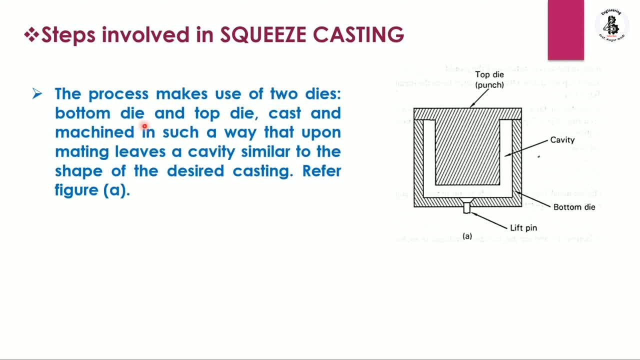 the process makes use of the two dies- bottom die and top die- cast and machine in such a way that upon the matting leaves a cavity similar to the shape of the desire castings. so this is our simple shape right now, but if you want to make a complex geometry, so you will also made then in second. 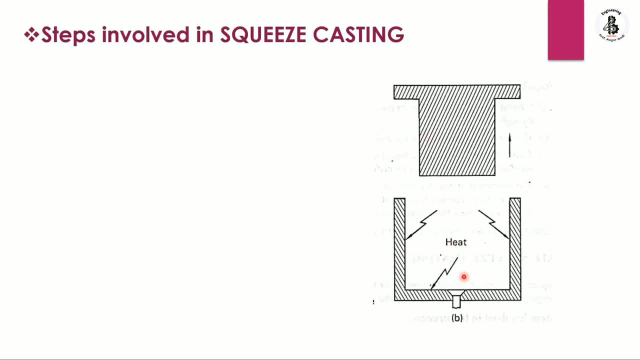 steps. just you can see: hit this bottom die and just you can see this is our top die. so what happens? the bottom dies is preheated to around 200 to 250 degree centigrade with the help of a torch and sprayed by a water-based. 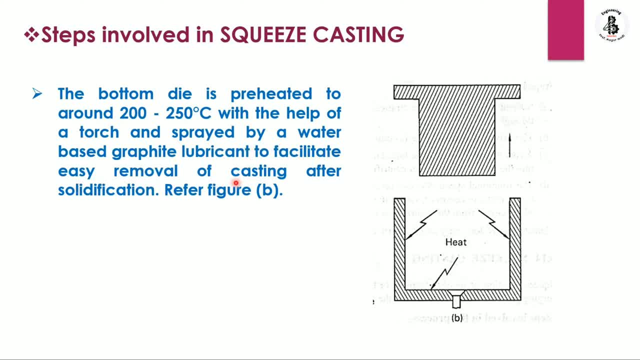 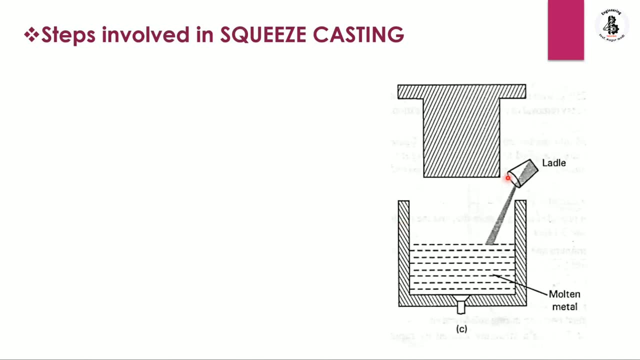 graphite lubricant to facilitate easy removal of the castings after the solidification process. so this preheating that will be essential in some applications for easily removing the components. then third steps. just you can see, with the help of ladle you should fill the molten form of the metal. 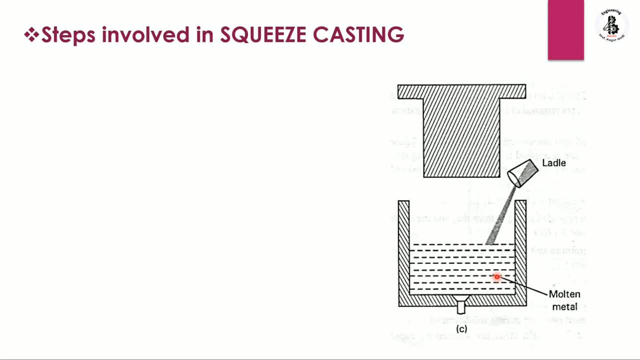 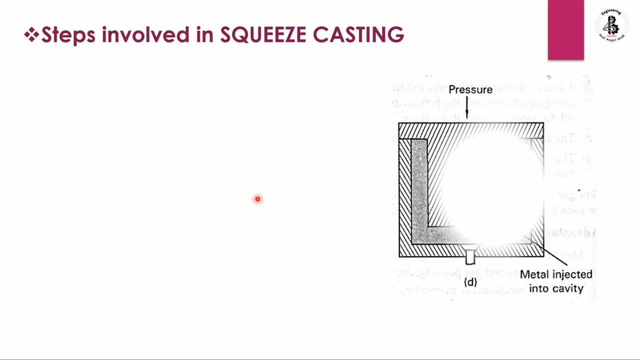 into this bottom die and after this, just you can see, the measured quantity of the molten metal is poured into the bottom die. so as the metal starts solidifying, then pressure is applied to the top die, causing it to move rapidly towards the bottom die. then just you can see. 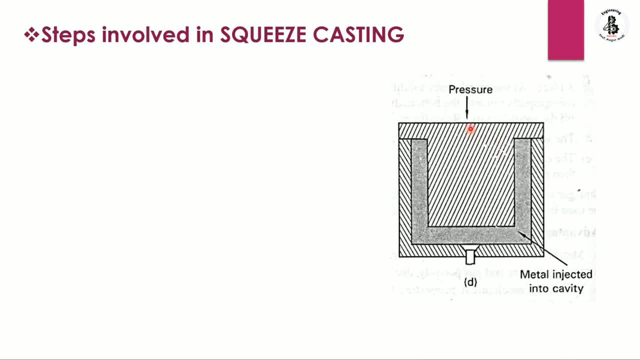 now this top die. it will be used to generating the pressure after some solidification process and this metal that will be solidified into that particular cavity. so this causes the molten matter to get squeezed and fill the mold cavity. the squeezing pressure is applied until the solidification is being completed. and last steps. 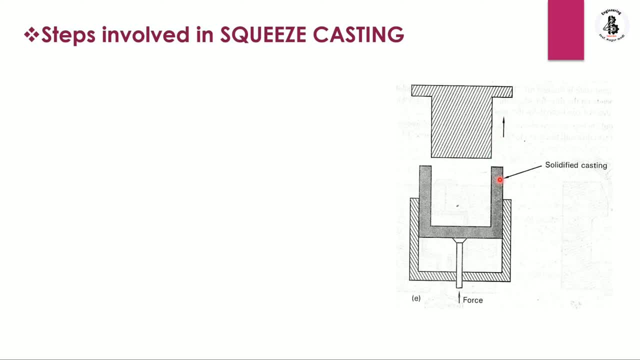 by the removing of the pressure with the help of top of die- this is, our solidified castings that will be my required shape and size of the job- and with the help of these ejector pins, applying the force so that will be easily removing of that. 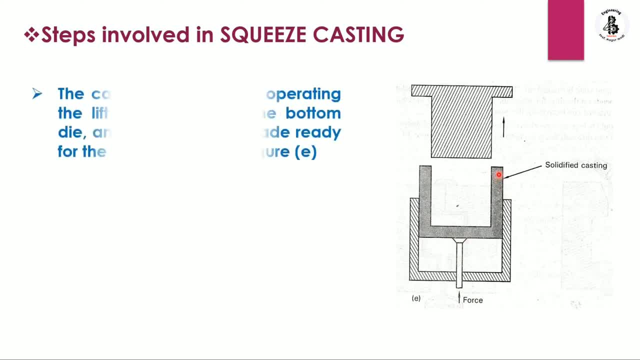 particular solidified components. so the casting is ejected by the operating lift pin provided into the bottom die and the die is then made ready for the next cycle. so you should repeat the cycle for the mass productions also. so this is the simple techniques for making a squeeze casting.